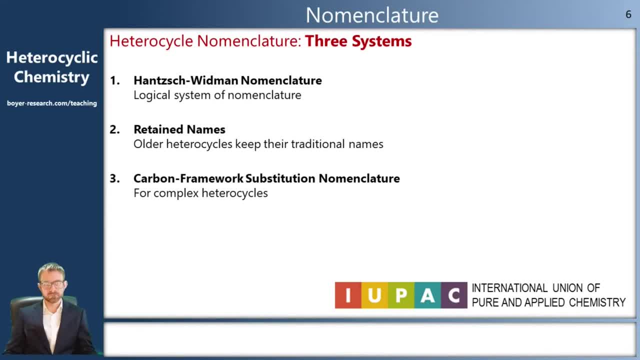 Chemistry? who is in charge of this kind of thing? The first set of rules is the Hans Wittmann nomenclature. This is a logical system by which you can name various different heterocycles. However, some of the older heterocycles which 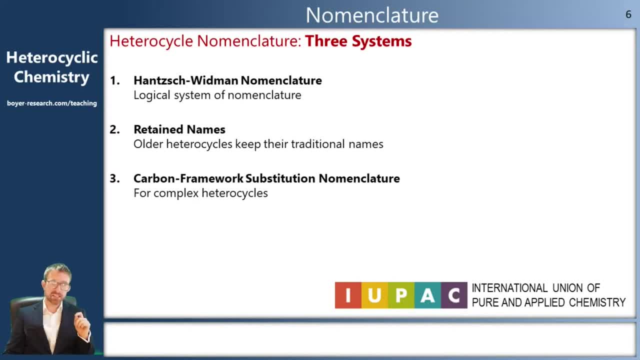 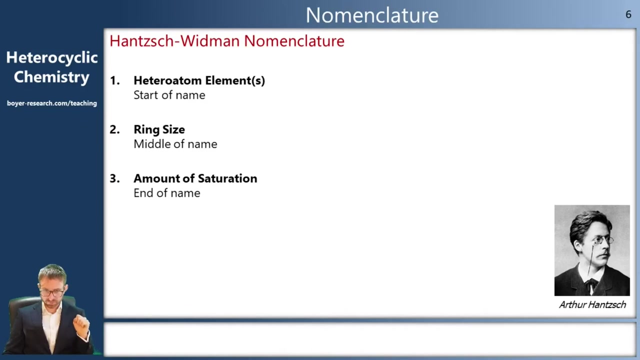 are very prevalent, keep their older, more traditional names. Finally, some heterocycles are very complicated and for those we need a backup system which involves naming the carbon framework and then describing where the heteroatoms are. So to start off with looking at the Hans Wittmann nomenclature in order to name a heterocycle, 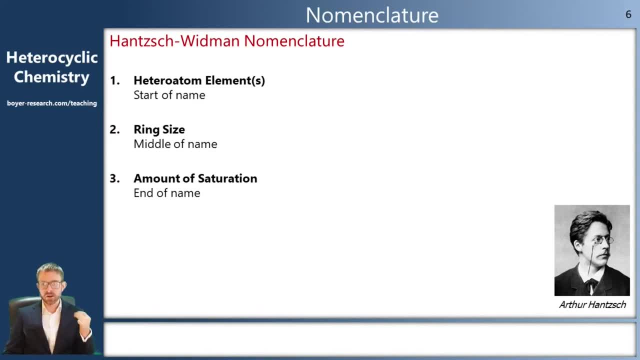 we really need to know three different things. We need to know what are the heteroatoms present in the ring, how big is the ring and how much saturation, how many double bonds are there in the ring? To make a name out of this, starting off with the heteroatom, we can use each element to 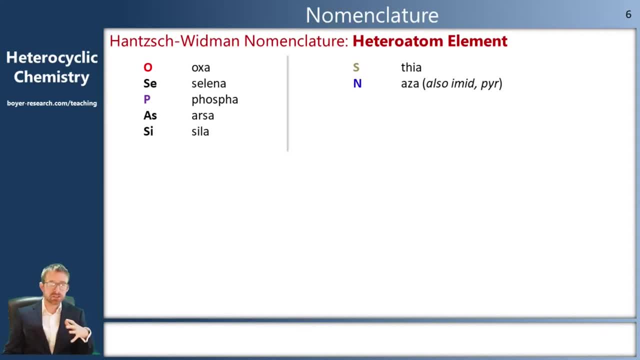 give us a prefix for the name. So oxygen gives us oxa, selenium gives us selenia, phosphorus gives us phospha, arsenic gives us arsa and silicon gives us silla. These are kind of obvious ones, but some of the other ones, such as sulphur and nitrogen, 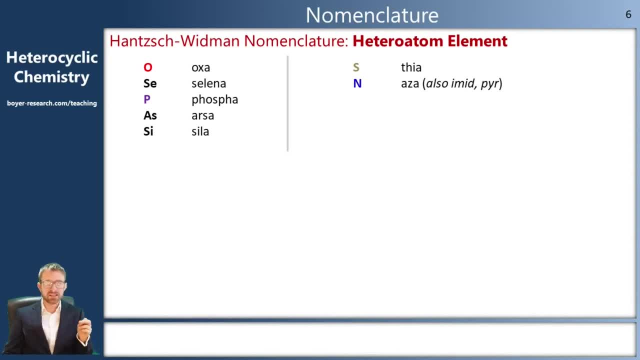 are a little bit less obvious. Sulphur gives us thia and nitrogen gives us aza, Although, as you can see, there are a lot of different names for each of these elements. For example, as you'll see, because nitrogen heterocycles are so important and prevalent, you'll see. 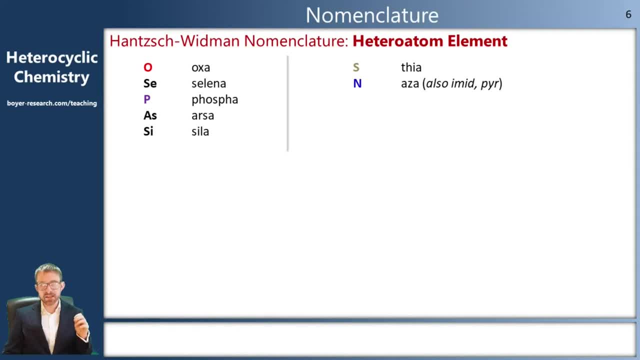 that sometimes, instead of aza, the prefixes imid and pir are also used. If we have more than one heteroatom in the ring, then we can use multipliers to describe the system. So one nitrogen, for example, gives us an aza molecule, but if there's two, 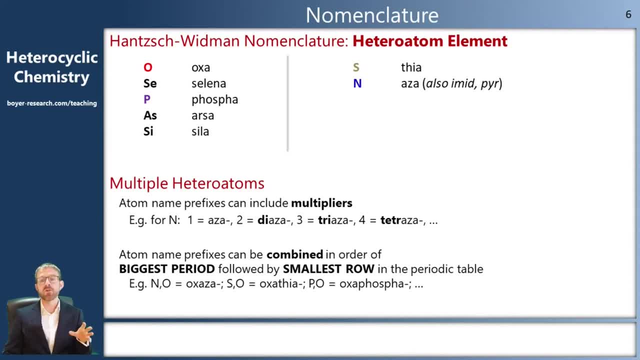 it's a diaza, If there's three it's a triaza, If there's four it's a tetraza Et-E-et. If there's two different elements in the ring, then we combine the two prefixes. If there's a nitrogen and a oxygen, it becomes oxaza. 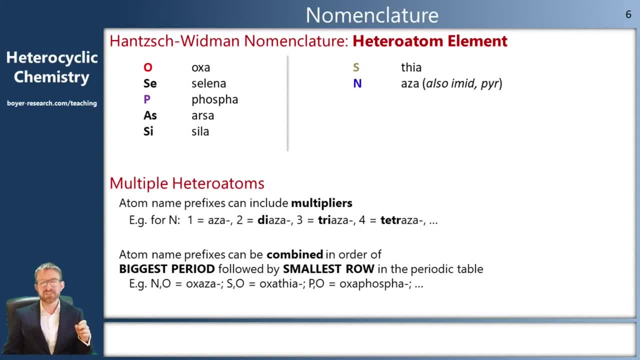 If there's a sulphur and a oxygen, it becomes oxathia. If there's a phosphorus and a oxygen, it becomes oxophosphate. Now The order in which we combine the names of oxygen and nitrogen and oxygen and oxygen. which element is furthest to the right, so has the biggest period on the periodic table. 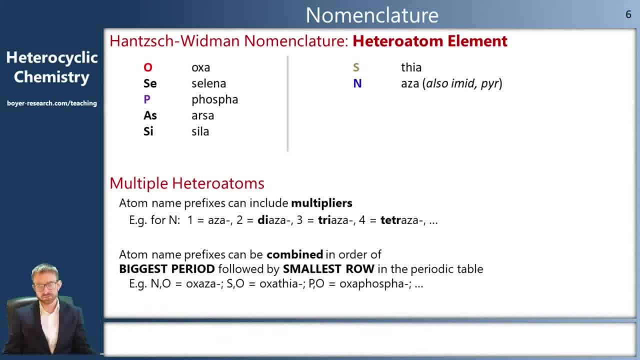 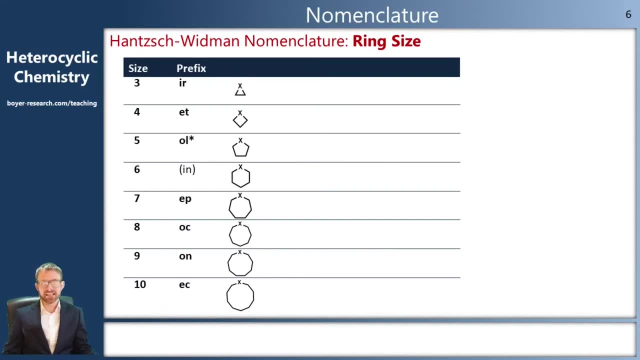 followed by which has the smallest row, so furthest to the top. Next, we need to look at the size of the ring in our heterocycle, and each size is given a different prefix. These prefixes are mainly derived from the Latin and Greek for numbers. 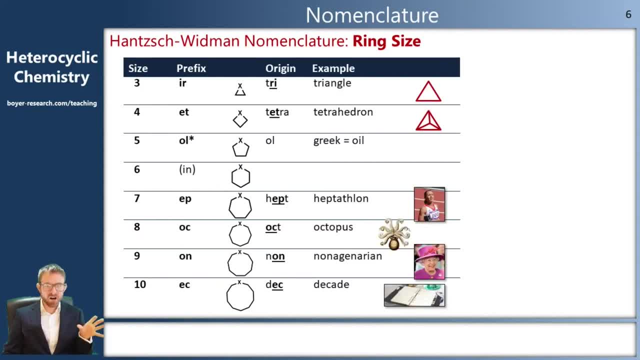 so, for example, 3-membered rings are IR and that's from the letters in tri as in triangle, but reversed. 4-membered rings are ET, from tetra, for example tetrahedrons. The 5- and 6-membered rings don't follow the rules, so 5 is OL and 6 is IN. 7-membered rings are: 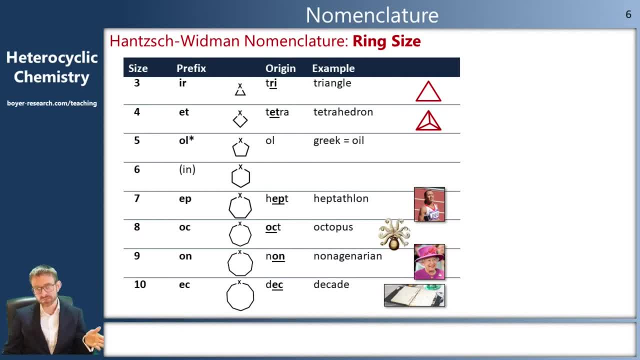 EP that's from hept, like a heptathlon. 8-membered rings are OC, from oct, like an octopus. 9-membered rings are ONS from non, as in nonagenarian, somebody who's 90 years old, And 10-membered rings are EC, as in deca, as in a decade. 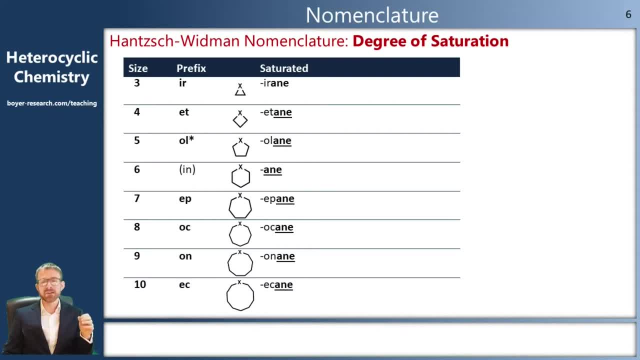 Finally, to make the last part of our name, we need to figure out how many double bonds there are. If the molecule is completely saturated, then we add the suffix ANE to the end of the name, so that 3-membered rings become IRANES, 4-membered rings become ETANES, 5-membered rings become 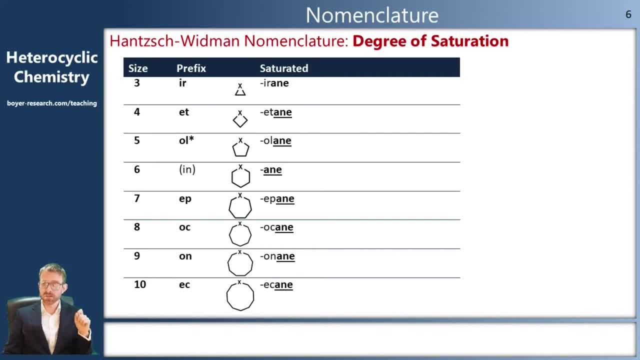 OLANES, Now 6. we lose the IN prefix for most of our rings, so they're just ANES, 7 are EPANES, 8 are OCANES and 9 are ONANES. So that's it. Thanks for watching. 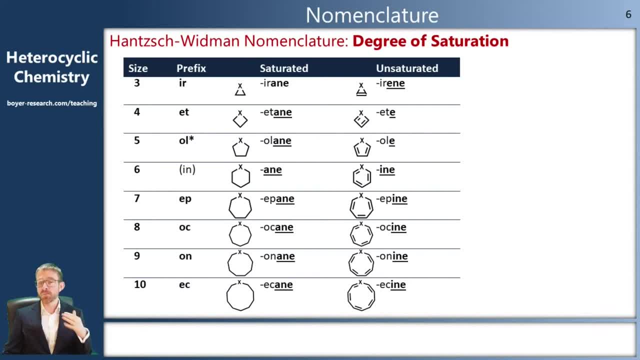 In the unsaturated version, so this is the version with as many double bonds as is possible. instead, we use the INE suffix. However, again, there are some exceptions, So we start off and instead of the INE we use ENE. So 3-membered rings are IRENES, 4-membered rings are EATS, so just an E instead of the. 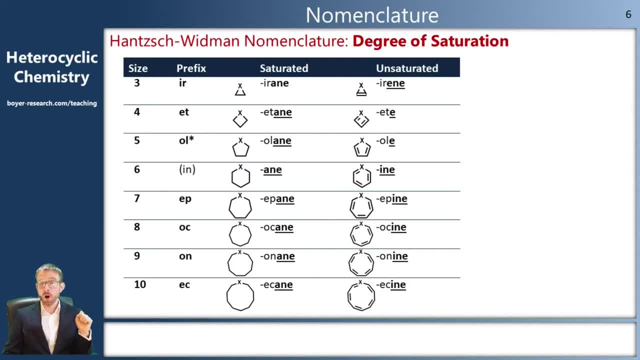 INE. 5-membered rings are OLES, so OLES instead of OLENES. 6-membered rings are OLEANS. 6-membered rings are OLEANS, So 4-membered rings are just EANS with no prefix. 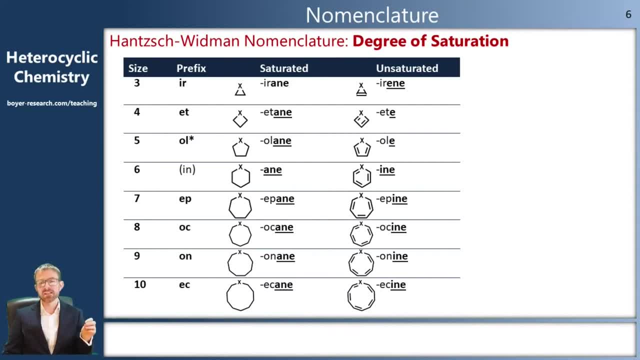 7-membered rings. We go back to the rules again, so it's EPIENS, OSEANS and ONEANS and ESEANS. However, Nitrogen gives us some problems, So for Nitrogens we use very slightly different names, and that are often names with an extra. 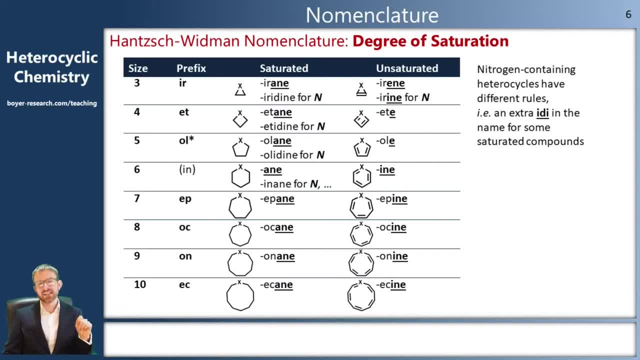 IDY in the name, So for 3-members it goes from instead of IRANE to an IRIDEEN. For four-membered saturated heterocycles it's an etidine for nitrogen. For five-membered saturated heterocycles it's an olidine. 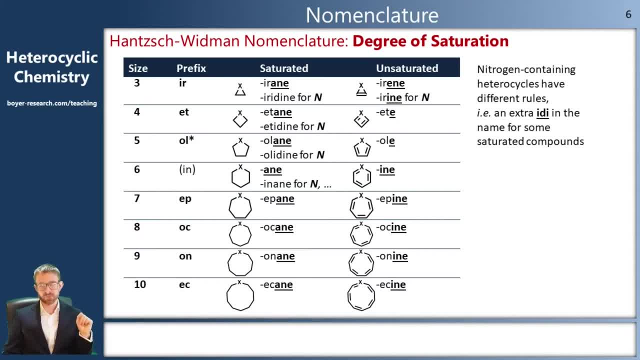 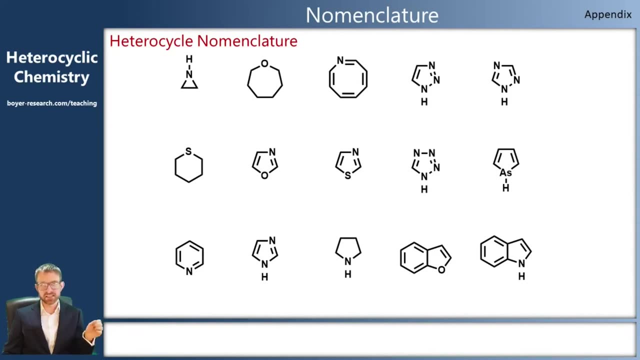 For six-membered heterocycles with nitrogen it's an inane. And finally, for three-membered unsaturated heterocycles with nitrogen, it's an irine, so spelled slightly differently. Looking at a set of heterocycles here, we can start to see how we can name these different ones. 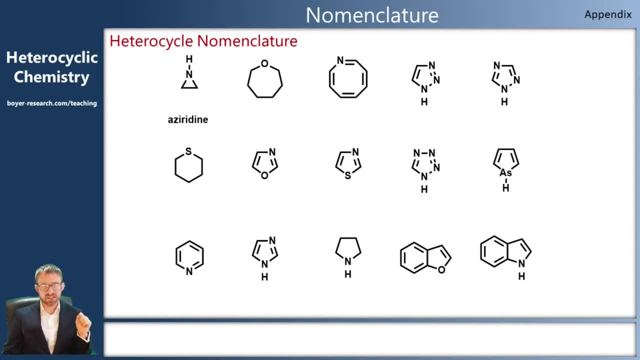 Our first one contains a nitrogen, so it's an, as It's a three-membered ring, so it's an ir. It's saturated with a nitrogen, so it's an idine, and that gives us an aziridine. Our next one is an oxygen-containing heterocycle, so it's an ox. 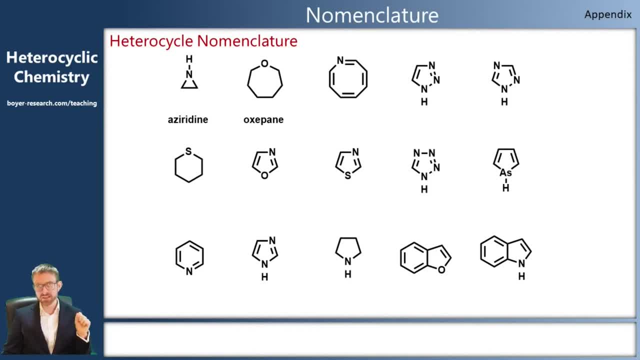 It's a seven-membered ring from hep, so we get ep. so that's an oxep. And again, it's completely saturated, so we get an a, so oxepane. The next example contains a nitrogen, so it's an as. 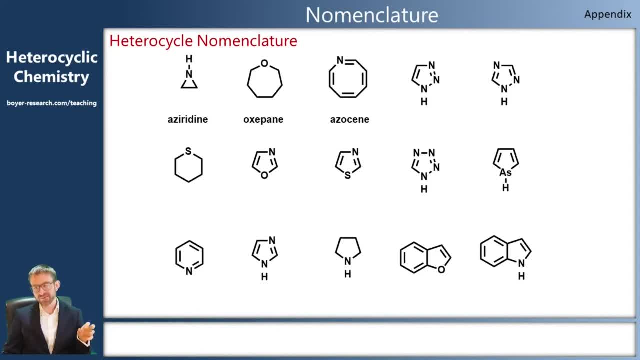 It's an eight-membered ring, so we look at octa or oc And now, because it's completely unsaturated, it's an ene which gives us an azocene. Moving on to our five-membered heterocycle, here we have three nitrogens. 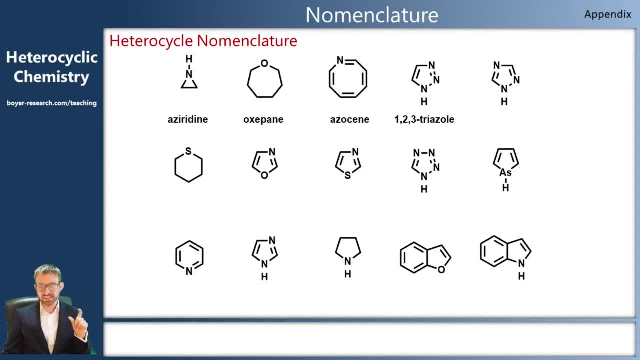 So because there's three, we can say tri Nitrogen is as, So it's a triaz and our unsaturated five-membered heterocycle gives us ol. So this is a triazole And you can see, in triazoles there are two different ways to put the nitrogens around the ring. 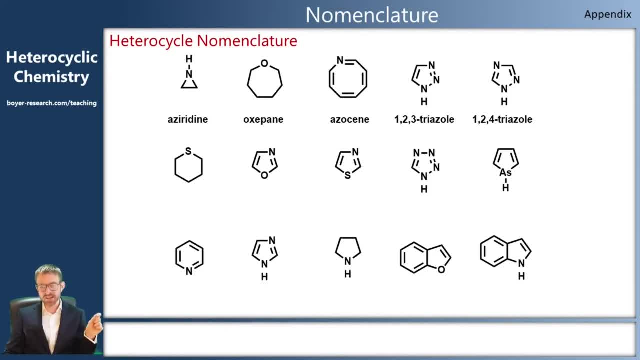 and we can differentiate those by using numbers. So one, two, three, where all the nitrogens are next to each other, and one, two, four where there's a gap. And we'll see more about numbering heterocycles later on. 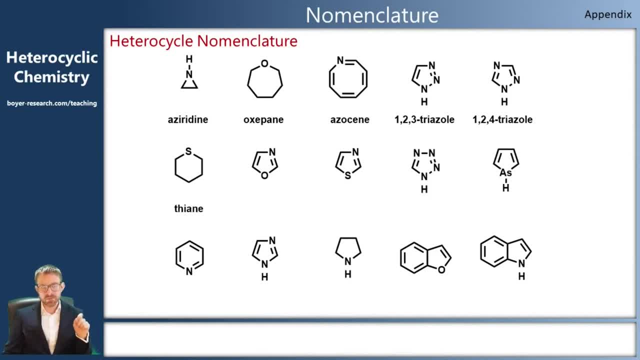 Moving on to the second row, we have a six-membered ring. It's containing a sulphur, completely saturated. This is a thiane. so thia for sulphur and ane for our six-membered saturated molecule. Now we have two heteroatoms- remembering to start, on the right-hand side, top of the periodic table. 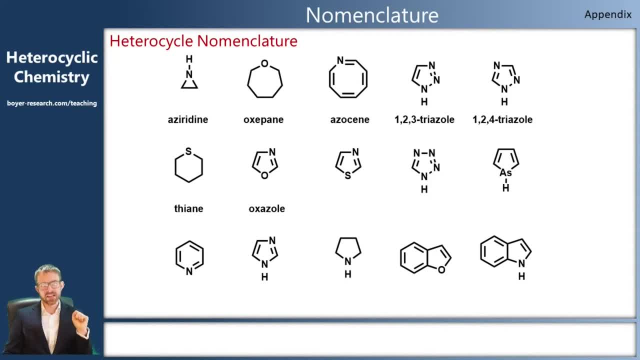 That gives us an ox for the oxygen, followed by an az for the nitrogen. It's a five-membered aromatic heterocycle. so that is an ol. So this is an oxazole. Similarly, instead of ox, it's an oxazole. 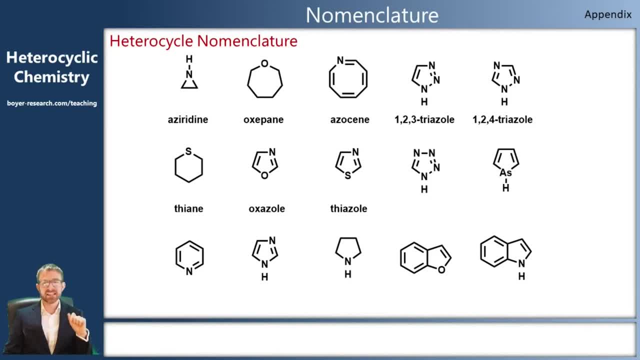 Now we have a sulphur, so we switch from ox to thia. That gives us a thiazole. This is again another ol, because it's a five-membered aromatic heterocycle. There is four different nitrogens in there, which gives us a tetrazole. 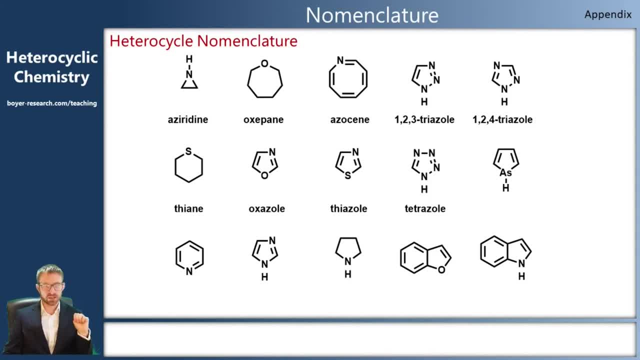 There's only one way to organise this, so we don't need to look at the numbers this time. And for the last one, again, it's an ol and the prefix for arsenic as well. You can figure this one out by yourselves. 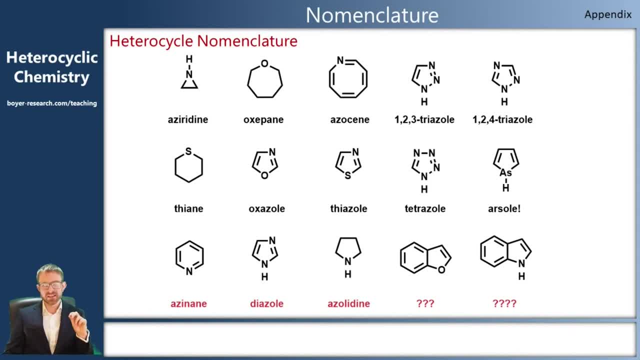 Well, we have some problems If we look at the bottom row of this. well, the names that we come up with here- so an azonane, a thiazole azolidines- don't actually correspond to the names we use for these heterocycles. 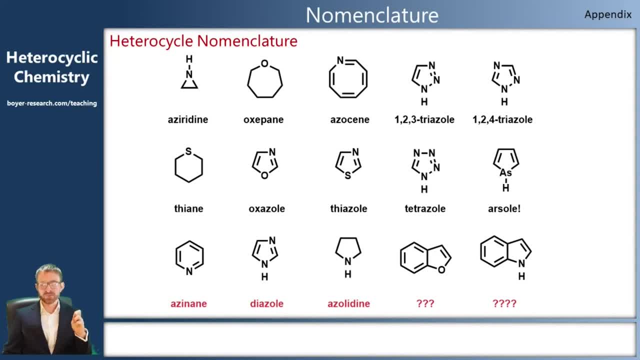 Furthermore, we have some complicated heterocycles down the bottom which we struggle to name in this system. So what do we do? Well, the ones on the bottom left all fall into the category of heterocycles with retained names. A lot of these are so important and well known. 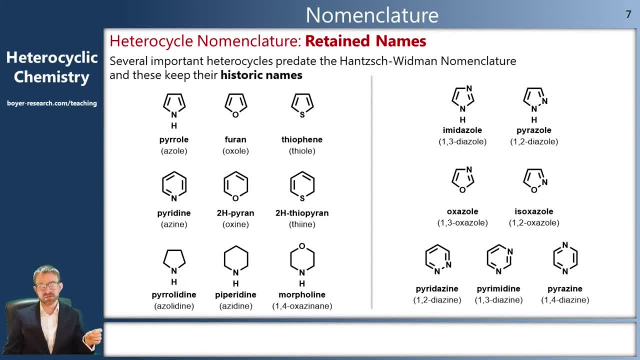 they actually predate the heterocyclic nomenclature system developed by Hans and Wittmann. So they're things like pyrrole and furon, which are known in ancient times, So pyrrole. again, this goes back to the element prefix. 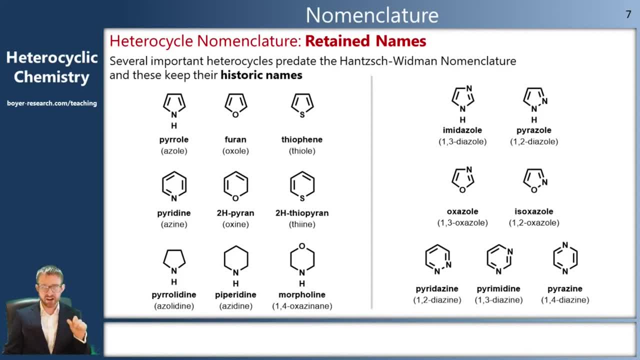 So actually the ol is correct. right, We have the right ole for a five-membered aromatic heterocycle, But instead of az, instead we use pyr. so this is a pyrrole Furon instead of an oxole. 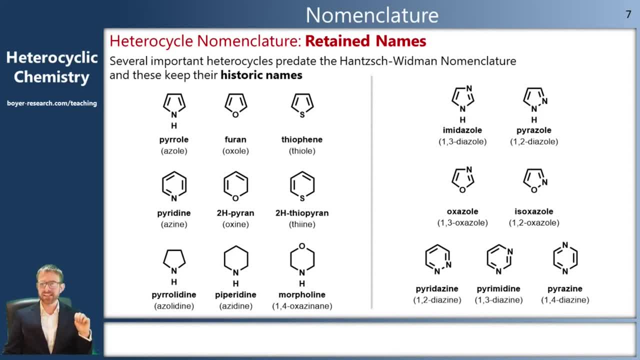 that comes from the fact that it's made from bran or furfur. in Latin We have a thiophene. instead of a thiol, We have a pyridine. So again we can see: instead of az, we're using the pyr prefix. 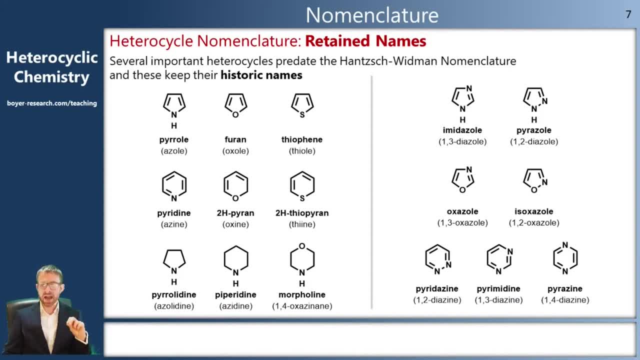 So we have a pyridine instead of an azidine, A pyrane instead of an oxine, A thiopyrane instead of a thylene. Pyrrolidine, again, is another one of our preferred names, as long as pyrperidine and morpholine. 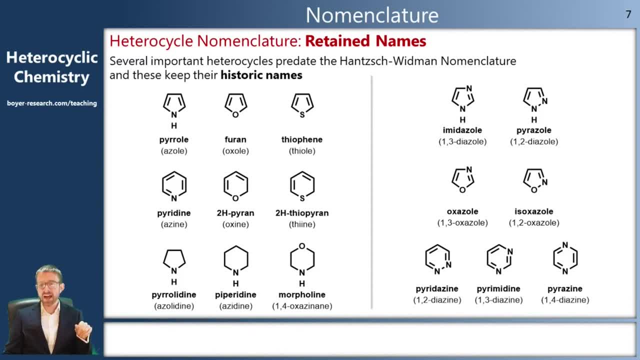 When it comes to heterocycles containing nitrogen and then another, or heteroatom, then again some of the names are retained rather than using the systematic approach. So, instead of calling the two nitrogen containing five-membered aromatic heterocycles, 1,3- and 1,2-diazoles, 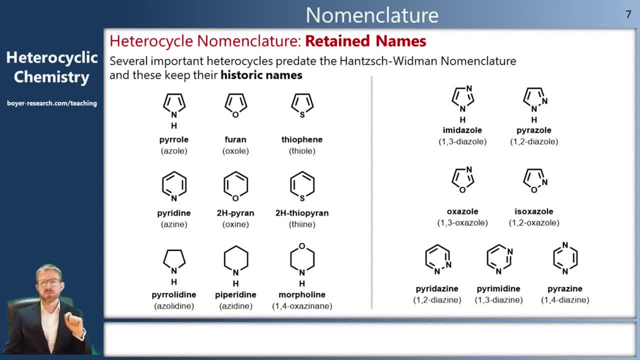 instead, we play around with our nitrogen prefixes. So the 1,3-diazole now becomes an imidazole and the 1,2-diazole becomes a pyrrozole, Now oxazole containing the nitrogen and the oxygen. 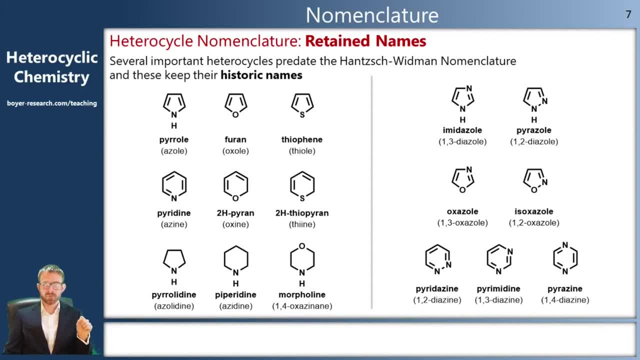 well, that follows the rules and it's actually a 1,3-oxazole, But instead of calling the 1,2-oxazole a 1,2-oxazole, that's called an isoxazole, And a similar thing happens to our six-membered aromatic nitrogen-containing heterocycles. 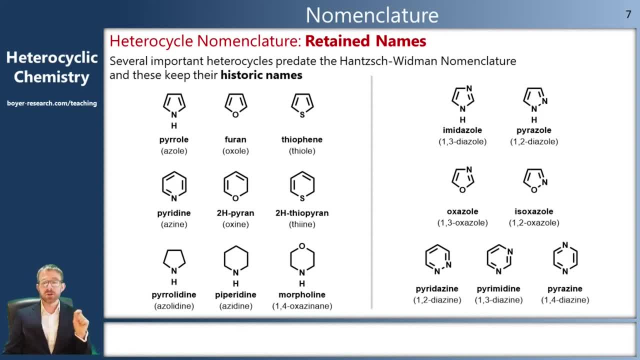 where we use two different versions of the prefixes for nitrogen to make the system. So the ene part gives us the correct name, but our system, with the 1,2-nitrogens next to each other, becomes a pyridazine. 1,3 is a pyrimidine. 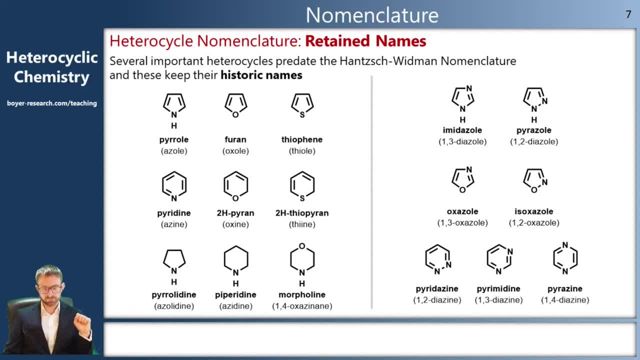 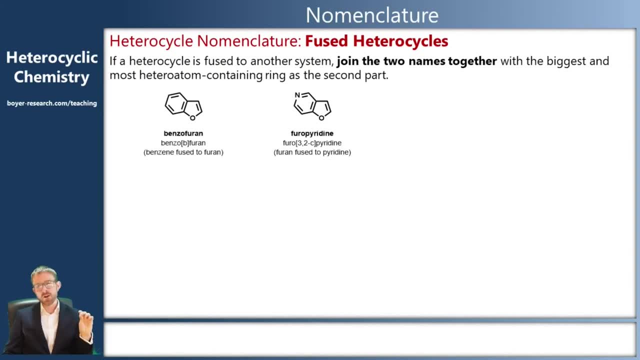 and the 1,4 is a pyrazine, But that still doesn't help us out with the two at the bottom right Now. these are fused heterocycles and actually, when it comes to fused heterocycles, so these are a furan fused to a benzene. 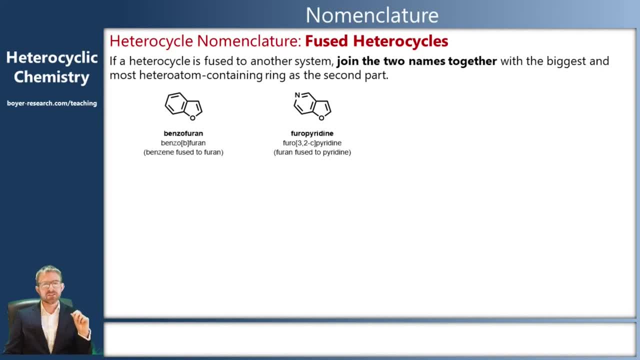 Well, we can just fuse the two names. So a furan fused to a benzene becomes a benzofuran, A furan fused to a pyridine becomes a furopyridine. The order in which we fuse the names means we take the biggest cycle that contains the most heterocycles. 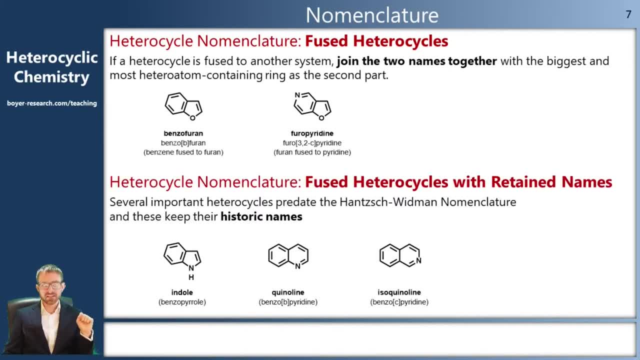 and that becomes last. Again, there are some fused heterocycles that have retained names. So instead of a benzopyrol we have an indole, and instead of benzopyrodines we have quinoline and isoquinone. 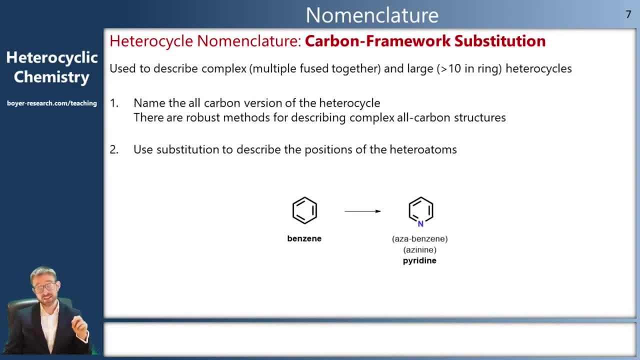 Now the final system. for very complicated heterocycles and heterocycles that contain more than 10 atoms in the ring, we have a system whereby we use the all-carbon version. Now the all-carbon version of names can cope with almost any different structure. 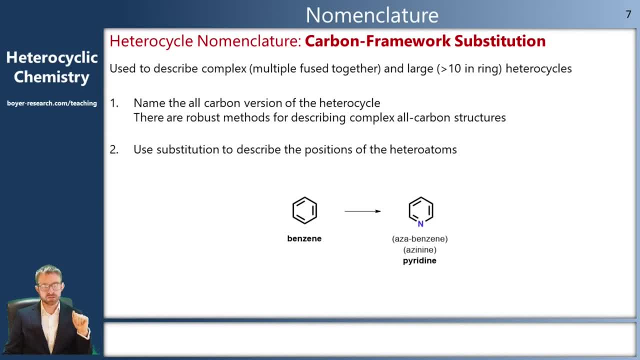 that has been conceived and therefore is extremely robust, And therefore what we do is we name the all-carbon version and then we'll just describe where the heteroatoms are. So, in a very simple example, benzene instead of becoming benzene. 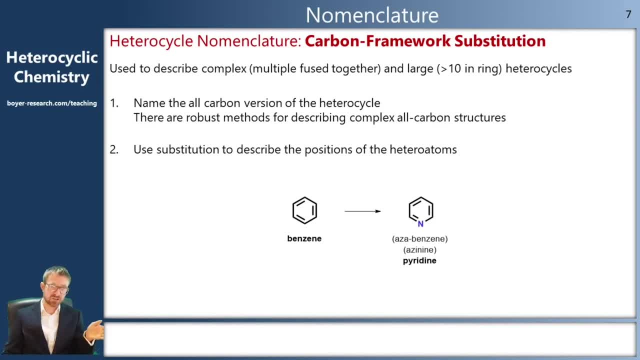 is an azobenzene, So it's a benzene. It's a benzene with an aza a and nitrogen in the ring. Of course we don't call that azobenzene. We don't call it azanine- the Hans-Richen rule. 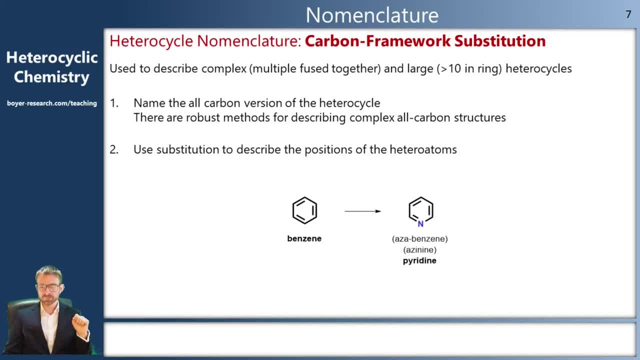 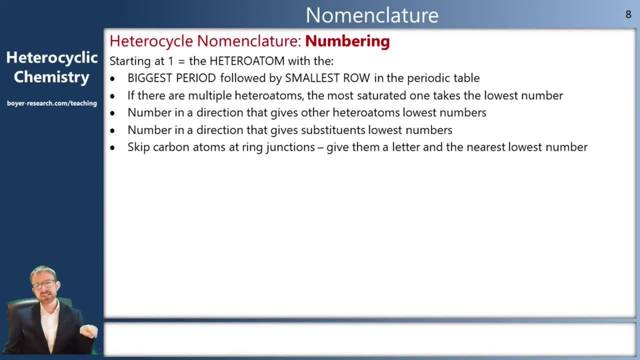 We call it pyridine from its retained name. When we talk about heterocycles, it's not just the heterocycles themselves, but substituents around the ring that are important, And therefore we need a system of numbering that tells us where things are. 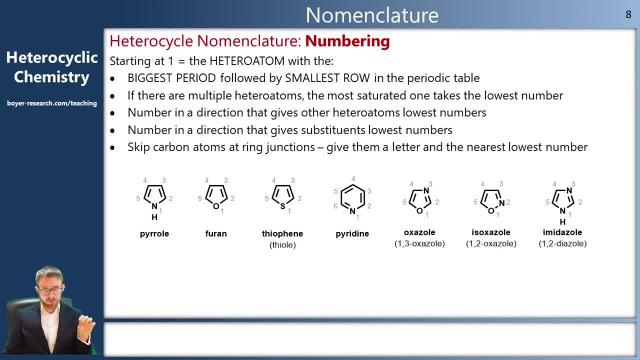 Now the system is simple. What we do is we start from the heteroatom that has the biggest period or the smallest row. so the same system as we used when we had the multiple heteroatom-containing molecules, and we call that one number one. 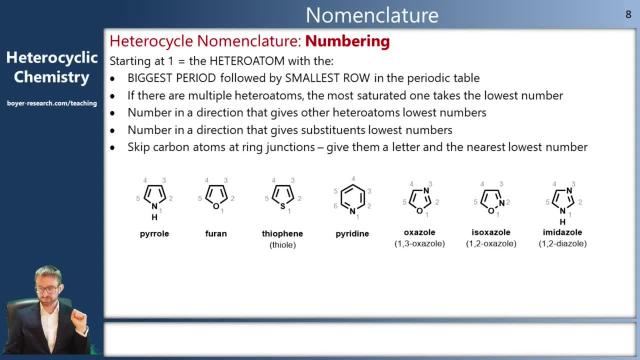 And then we number around the ring consecutively. Now, if there's more than one heterocycle, we want to number around, so we get the next heterocycle, like in oxazole becomes the lowest number. So this is a 1,3-oxazole and not the 1,4-oxazole. 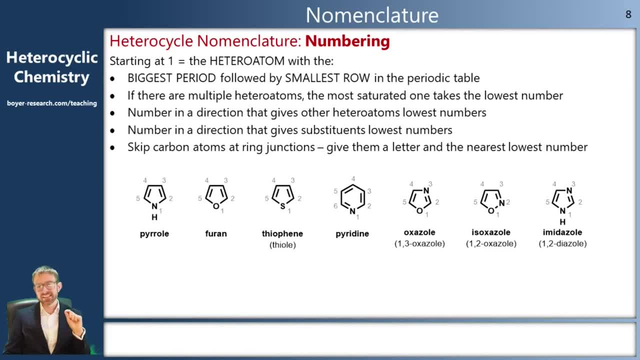 If there were two nitrogens in the same ring, like in an imidazole, the one which is most saturated has the lowest number. So the NH is N1, rather than the other one, the N3. We also, when we do numbering, we want to try and get any substituent. 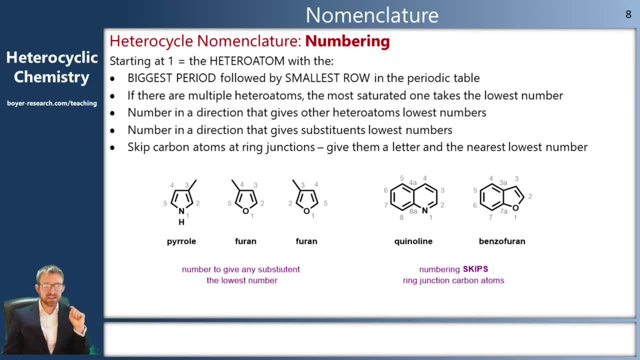 to be the lowest number. So in the first example we have a 3-methylpyrrole. that's fine. But in the second one we've kind of drawn a 4-methylpyrrole, but we don't really want that. 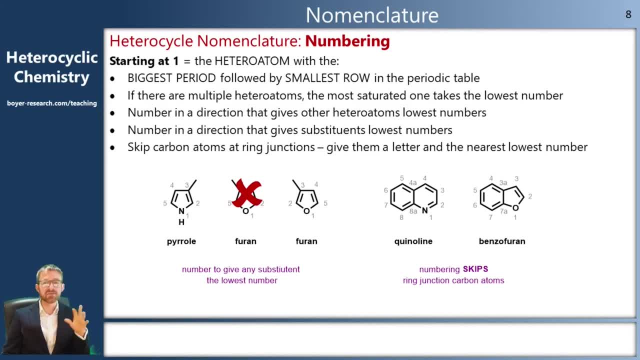 It's a much lower number if we call it a 3-methylpyrrole, and it's the same compound. Now, when it comes to fused molecules, we use the same system. We start from the heteroatom, we number around the ring. 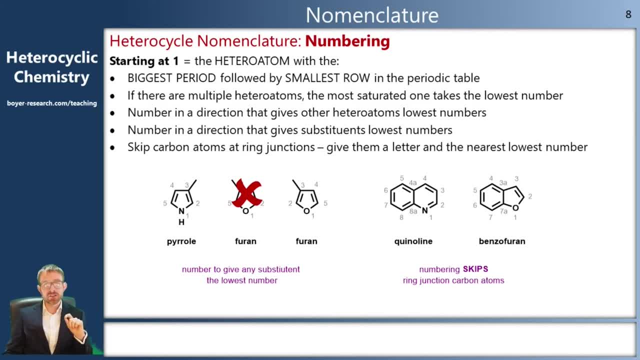 But what's important here is that we miss out any of the ring-junction carbon atoms. So you can see here quinoline starts off. nitrogen is 1.. The carbon next to that is number 2.. The carbon next to that is number 3.. 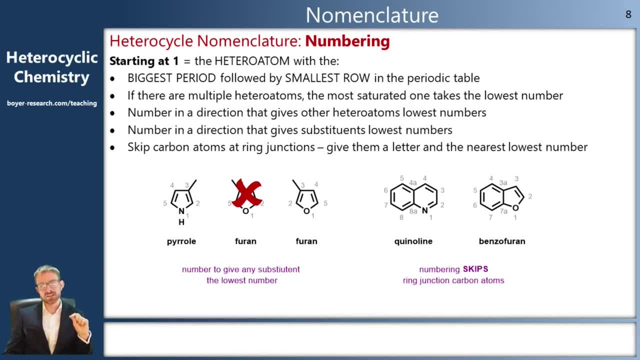 Then number 4.. Now the next carbon round is at the ring-junction, So instead of being called 5,, that becomes 4A. We skip that one and we carry on 5,, 6,, 7,, 8.. 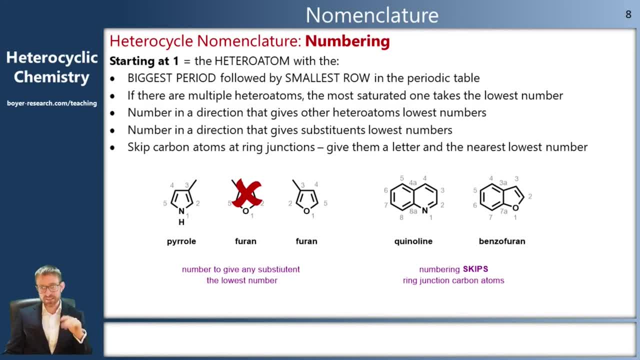 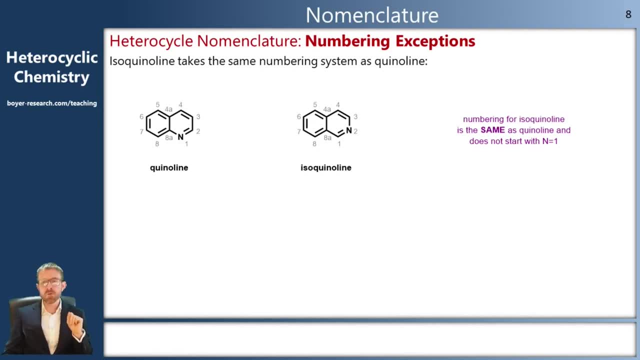 And then the last one becomes 8A. The exact same system can be applied for benzofuran. Finally, just because there wouldn't be a rule unless there was an exception, one of our retained named heterocycles, so our isoquinoline. 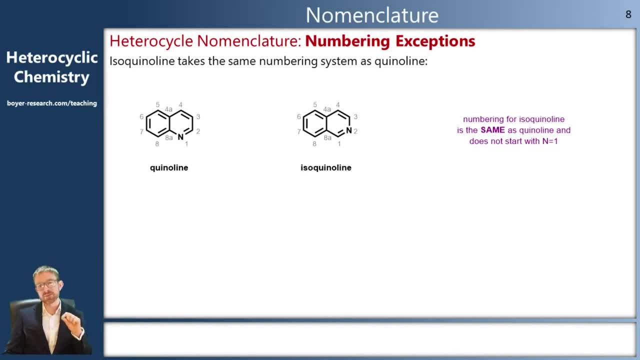 doesn't use the same numbering. The system where we'd expect to start the number at nitrogen being 1, it uses the same numbering system as quinoline, So be careful with this one. the rest of them are all fine. 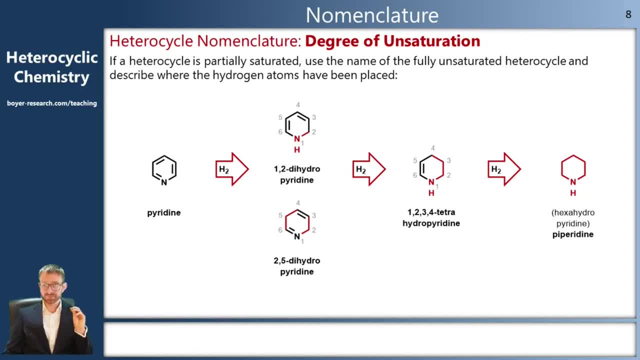 So, finally, we need to think about what happens when we have partial hydrogenation. Our system tells us how to name compounds like pyridine, which are fully aromatic, or like piperidine, which are fully saturated. So what happens in the middle? 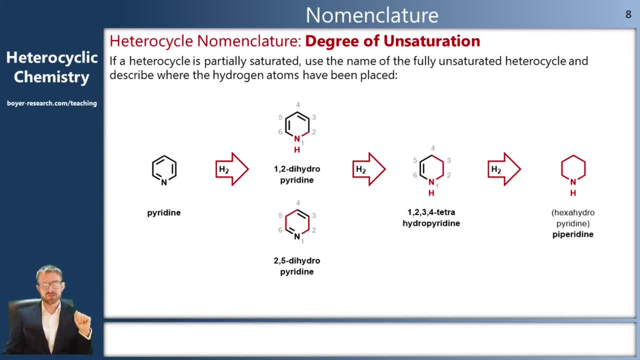 Well, here we just use the numbers to describe where the hydrogens have gone. So, for example, if we take pyridine and we put two hydrogens on, well, there's two ways we can do that. We can put the hydrogens at the 1, 2 position or the 2 and 5 position. 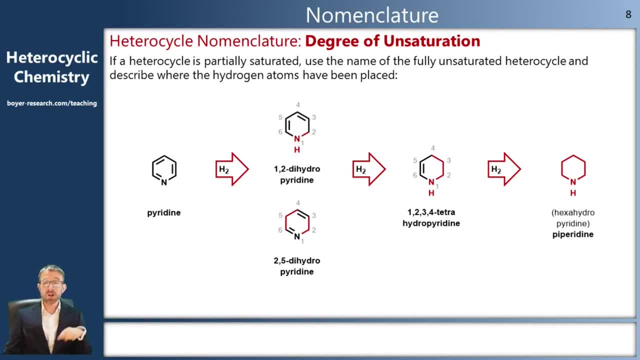 So these molecules become dihydropyridines. We can go one step further and we can get tetrahydropyridines. Now, obviously, when we go all the way to the next stage, we get hexahydropyridine, which we call epiperidine. 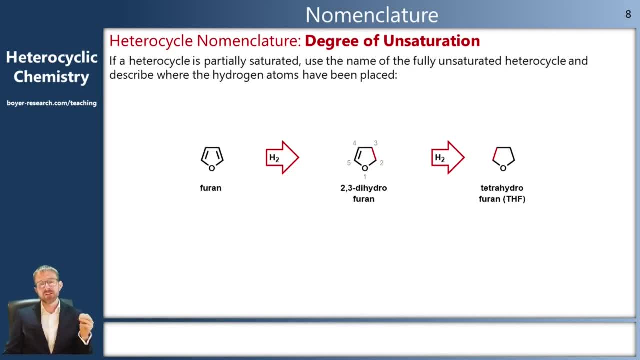 We can do the same thing with furan, where furan starts off as a furan, then goes onto a dihydropyridine, again using the numbers to describe where the hydrogens are finally getting tetrahydropyridine or THF. 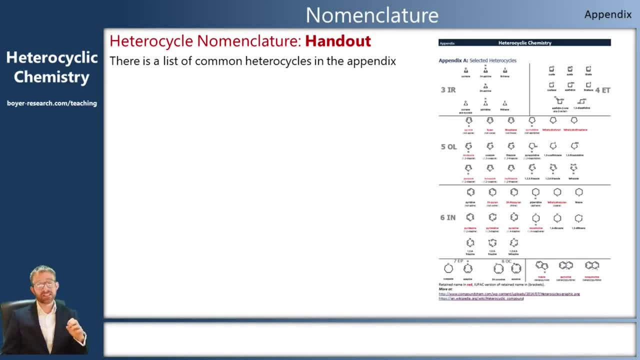 So I've tried to walk us through the different systems used for naming heterocycles. I've also compiled a list of the most commonly encountered heterocycles in the handout, if you prefer, just to learn them, which is a perfectly acceptable way. 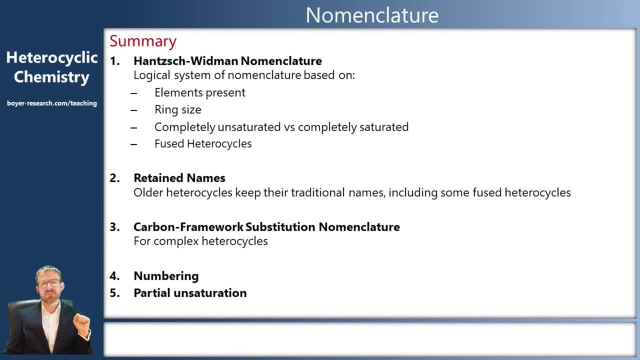 In summary, there are three systems for naming rings. We have the Hans-Wittner nomenclature, which is a logical system based upon the element's presence in the ring, the ring size and how saturated or unsaturated this molecule is. 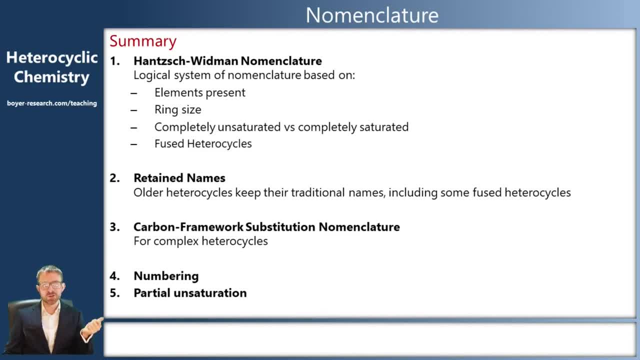 We can see. that also helps us name fused heterocycles. And But some of our older heterocycles, some of the more important ancient heterocycles, keep the original names, the ones that they had before Hans-Wittner nomenclature came along. 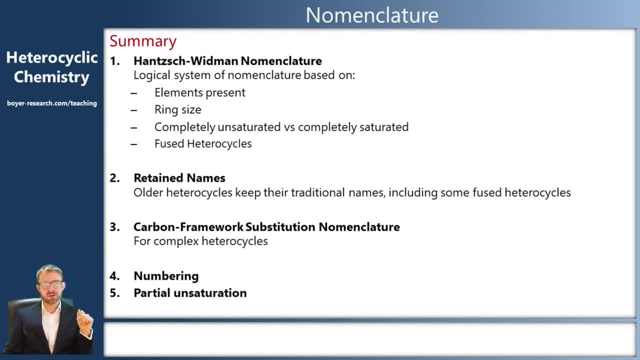 Finally, when things get too complicated, we have to use our carbon framework substitution nomenclature. We've also seen how we can refer to the different positions on heterocycles by numbering and what happens when we have a partially saturated heterocyclic system. Thank you for watching. I'll see you next time.